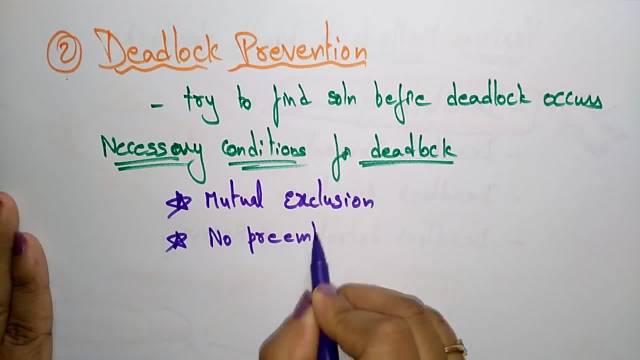 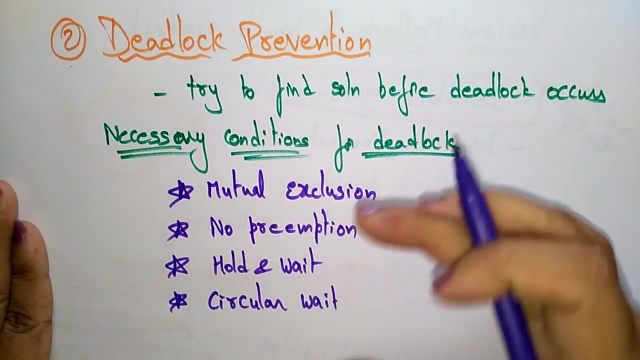 And next: no pre-emission. No pre-emission will leads to deadlock. Hold and wait condition: Hold and wait resources leads to deadlock. And next is a circular wait, Circular wait. So these are the four conditions, the four main conditions that leads to a deadlock. 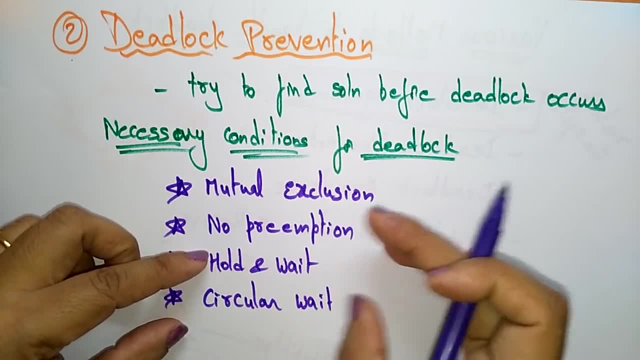 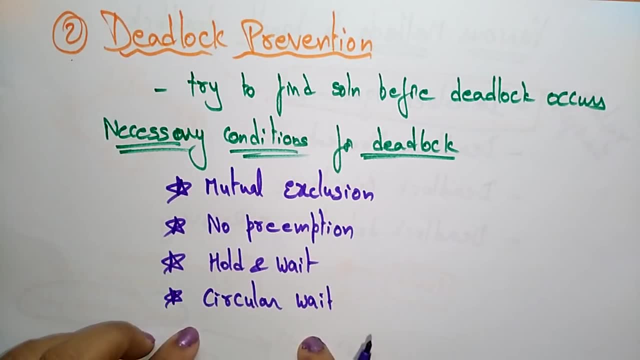 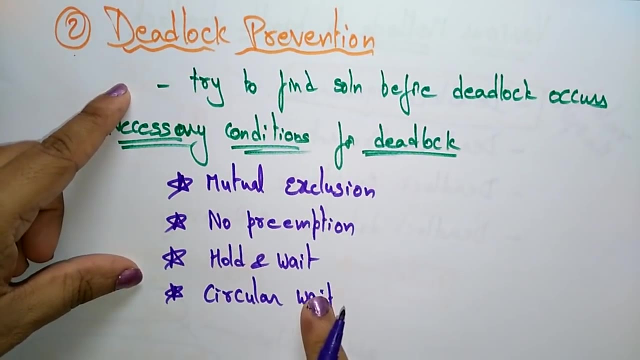 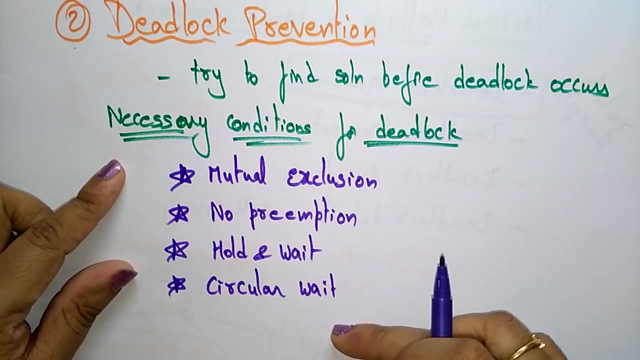 If all these situations are true, obviously deadlock will occur. Whenever the mutual exclusion is true, deadlock occurs. No pre-emission deadlock, Hold and wait. Circular wait leads to deadlock. Deadlock prevention says what this deadlock prevention says. the deadlock prevention says: either try to remove all the four conditions, try to make all the four conditions false, or at least try to remove one of the conditions or make at least one of the condition false. 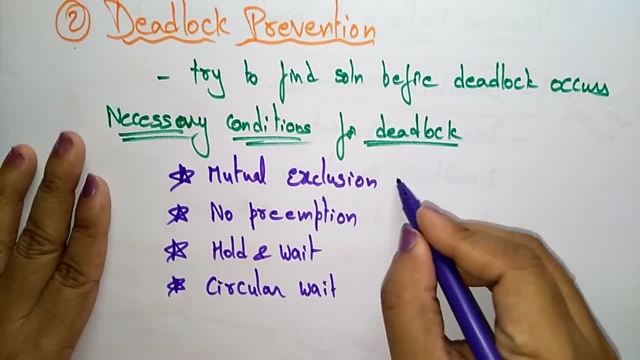 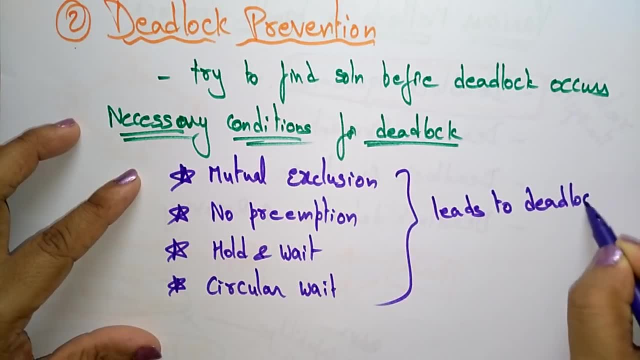 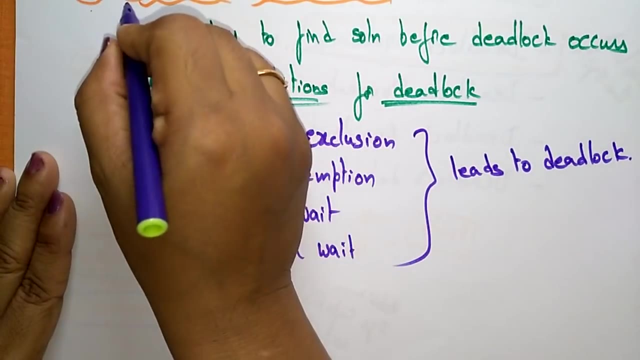 That leads to deadlock prevention. The first thing is, these four leads to deadlock. Deadlock Leads to deadlock. Okay, Mutual exclusion, No pre-emission. Hold and wait, Circular wait leads to deadlock. So then, deadlock prevention. what this deadlock prevention is saying. 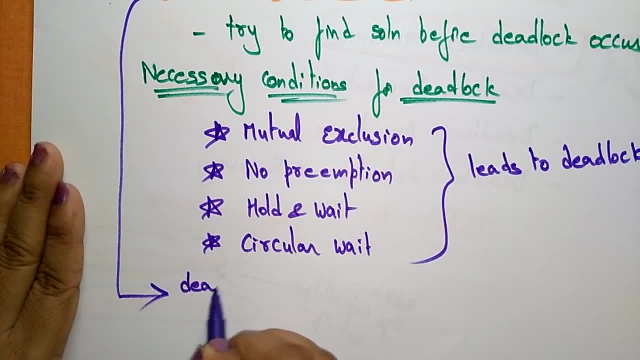 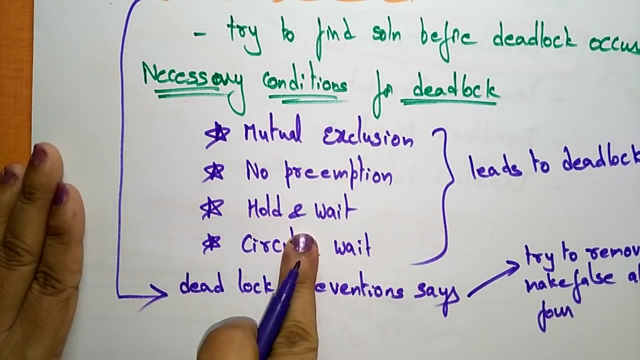 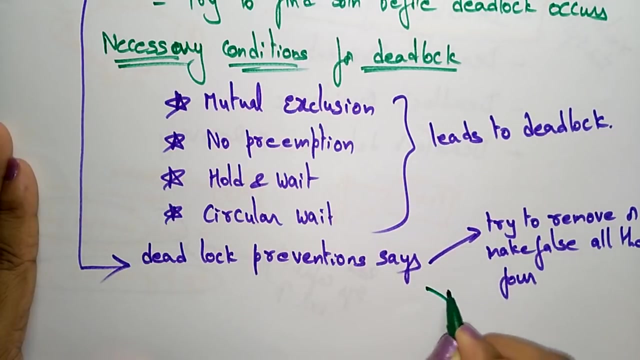 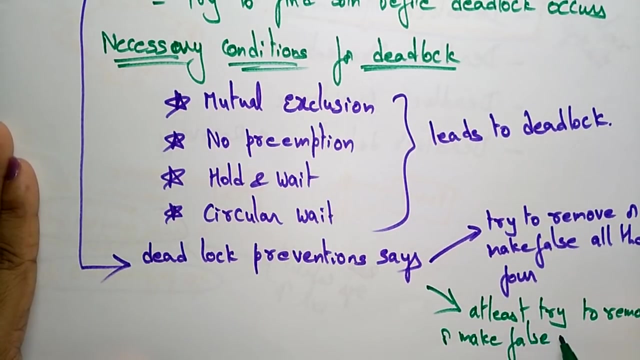 Deadlock prevention says. Deadlock Prevention Says: Try to Remove Or make false all the four conditions, all the four conditions. try to remove or make false all the four conditions, or or at least at least try to remove or make false any one of the condition, any one of the condition. then your deadlock can. 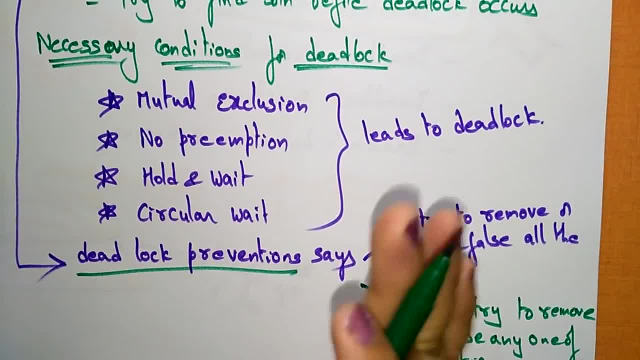 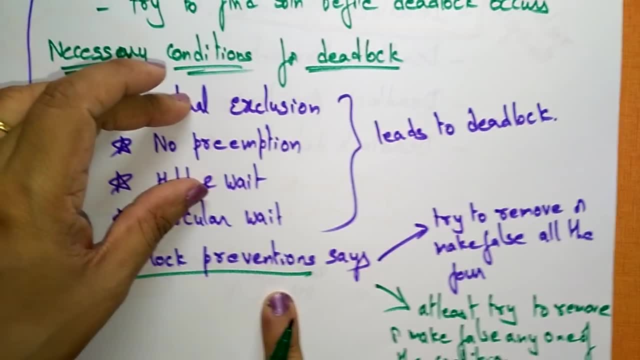 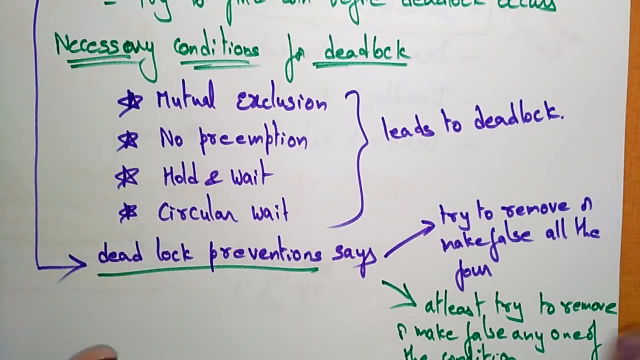 be prevented. so the main solution for this preventing is try to make all these mutual exclusion false, no, a permission false, hold and wait and circular, wait or false, okay, or or try to make any one of the condition as a false. if any one of the condition is false, then the deadlock will be prevented. so how? 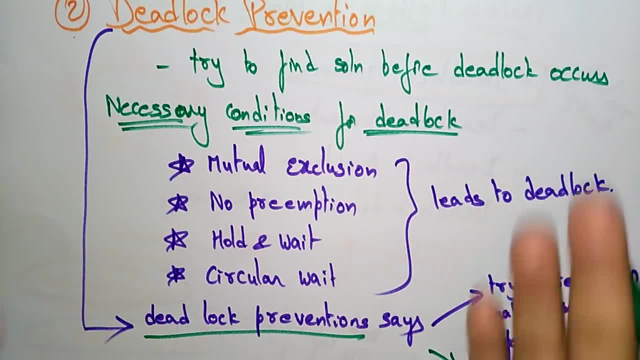 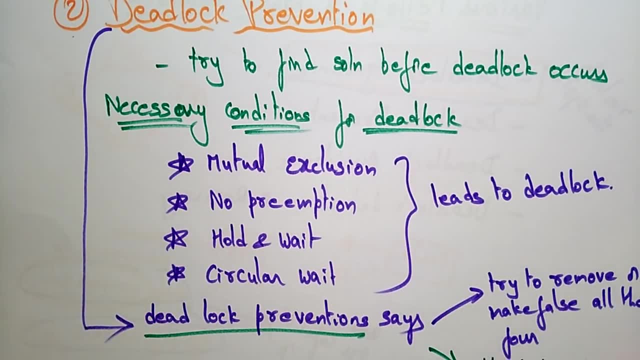 what is that? what is? how can I make mutual exclusion false? how can I make no preemption false? how can I make hold and wait, no, hold and wait, no circular wait. how is it possible? now, let us see that. so first let me take, let me try to. 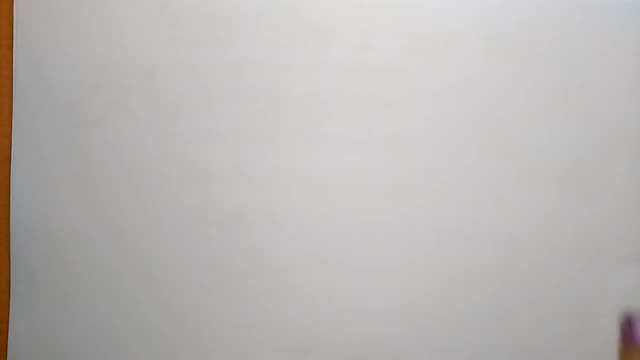 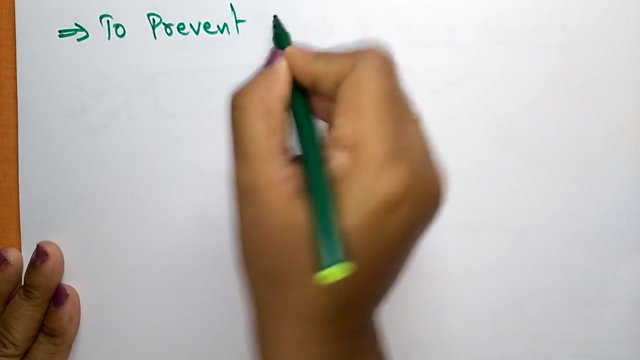 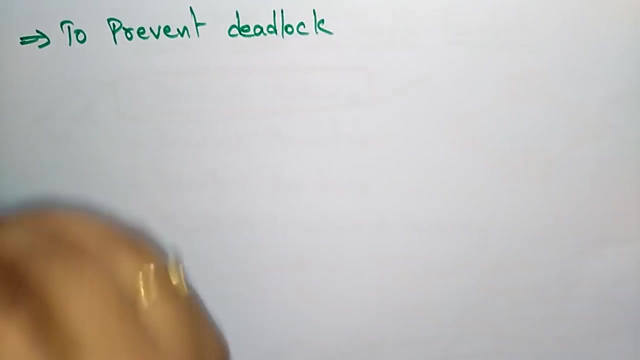 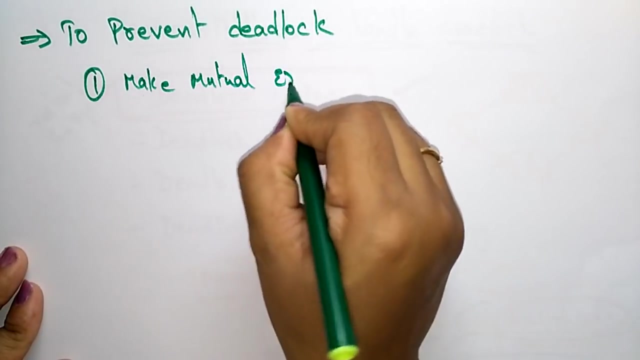 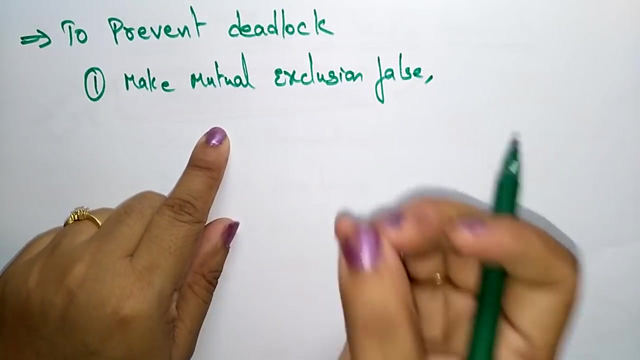 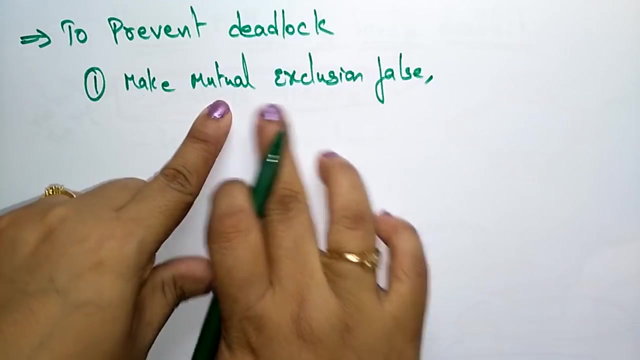 explain about the deadlock to prevent deadlock. to prevent deadlock. okay, to prevent deadlock, first make mutual exclusion false. make mutual exclusion false. mutual exclusion means what is mutual exclusion means the same resources. the process is a different process of sharing the same resources means the sharing concept is a mutual. no, sharing concept is the mutual exclusion. 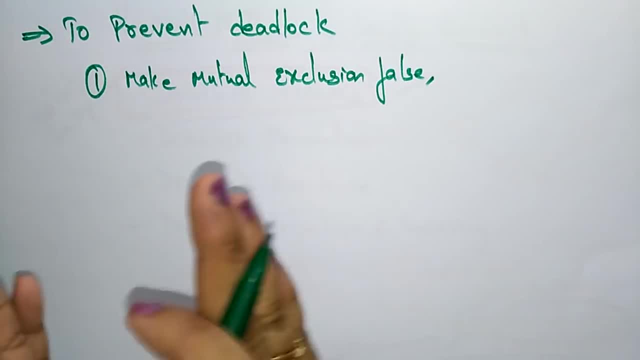 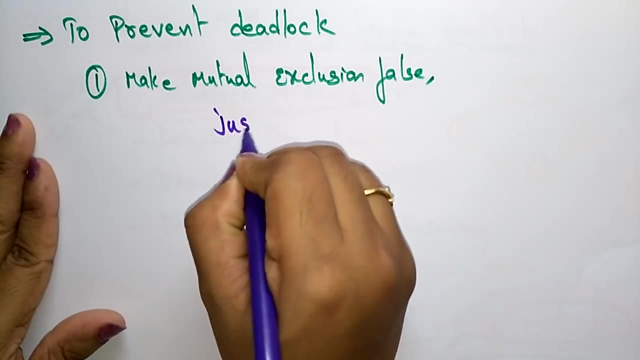 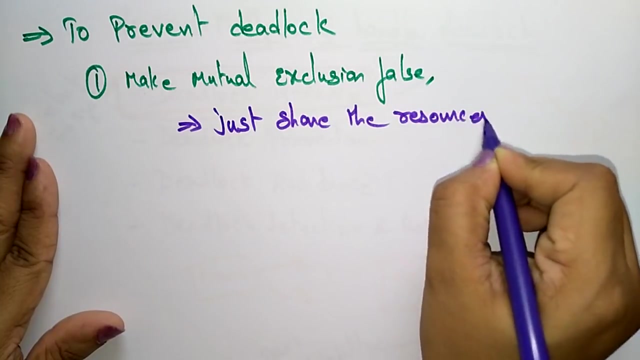 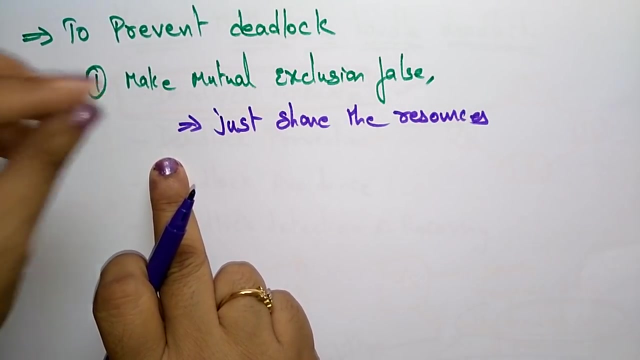 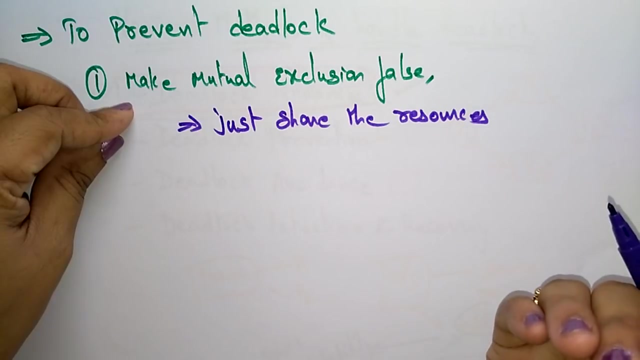 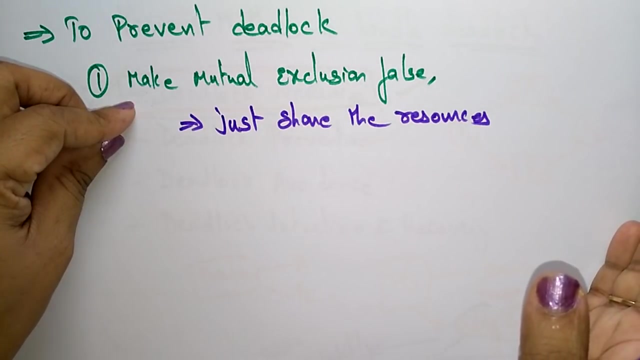 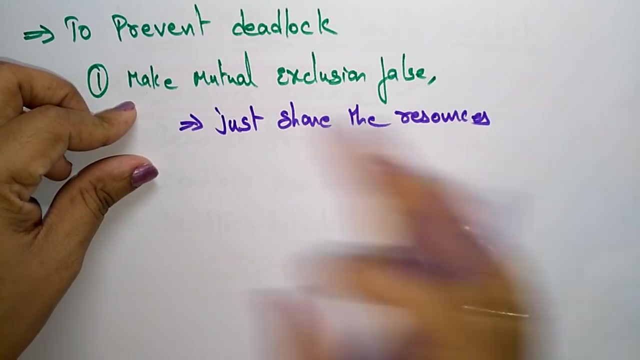 So you have to make the share. So let me explain it: Make mutual exclusion false. How can we do this? Just simply just share the resource. So the one way to prevent the deadlock is: first I will talk about the mutual exclusion First- make the mutual exclusion false. Whenever the mutual exclusion is false, the deadlock can be prevented. How can I make mutual exclusion false? Just share the resources. If the resources is sharing by every process, there is no mutual exclusion concept. Mutual exclusion means each process, one process after the another process. There is no sharing concept. 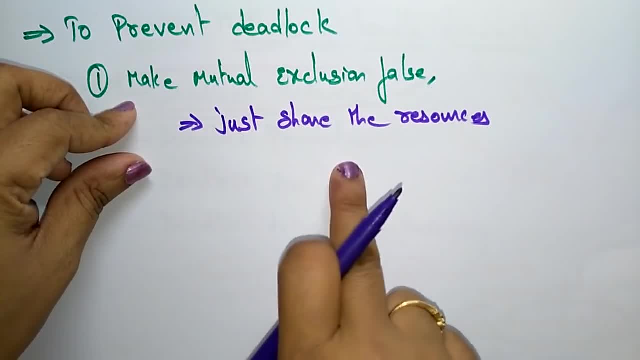 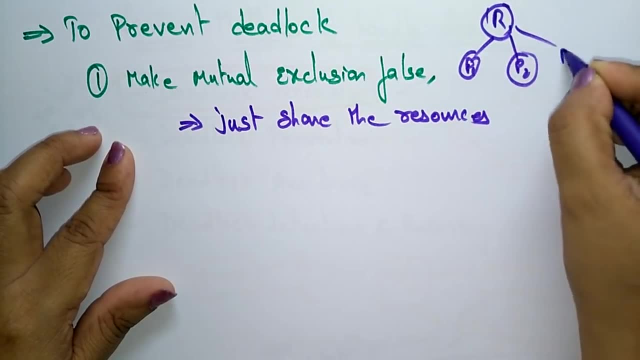 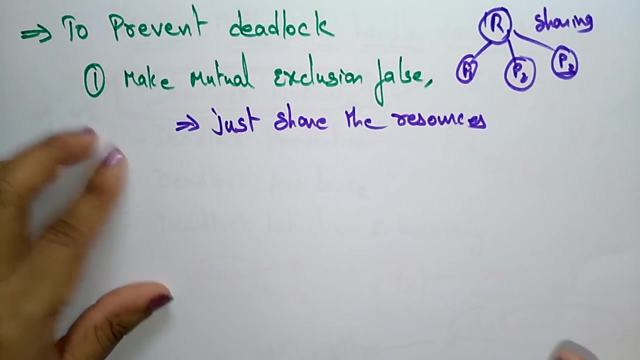 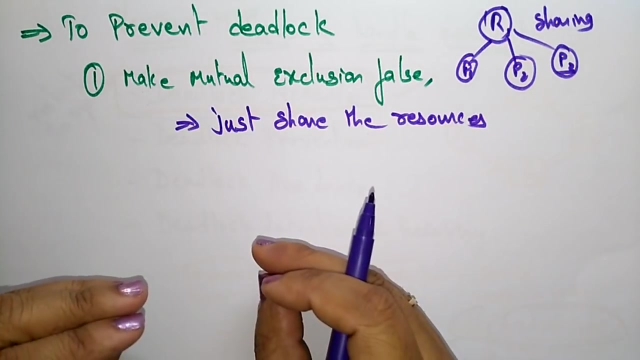 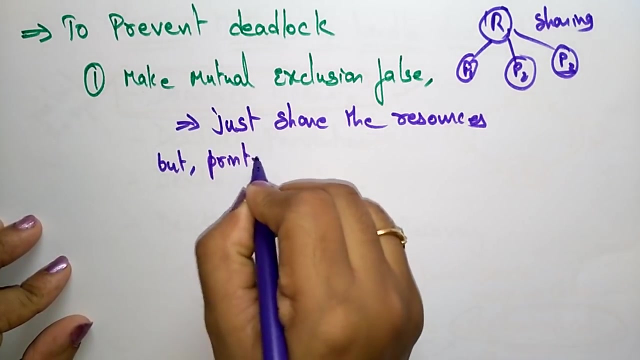 So if you share the resources, this becomes the false. Then if one resources is sharing by All the process- P1, P2, P3, then there is no deadlock. If sharing is there, there is no concept of deadlock. So try to make mutual exclusion false. But is it possible? But it is. in some cases it is possible. But it is not possible in the case of printer, Because printer is a non-shareable. 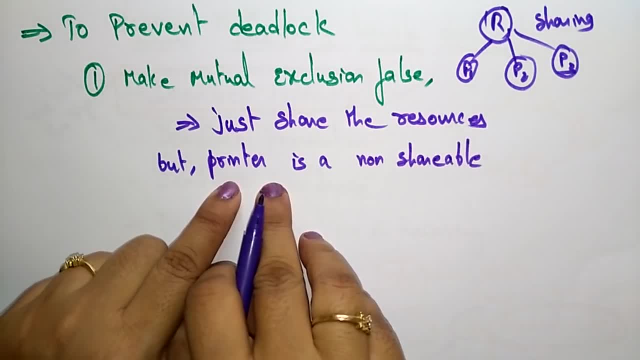 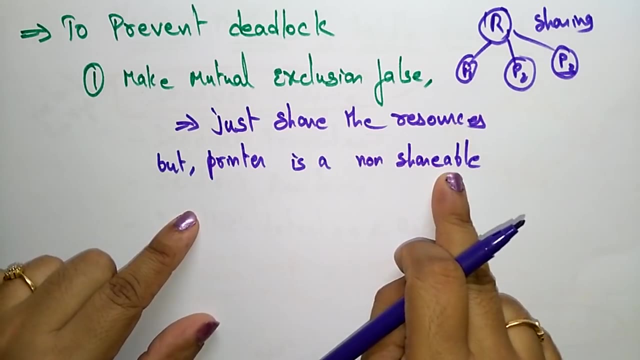 So for printing, one process will first print one page. Another process requesting process that will be print after the completion of this page only, So that printer can not share by every process Means at a time. So printer is not shareable. So this concept will not mostly work. 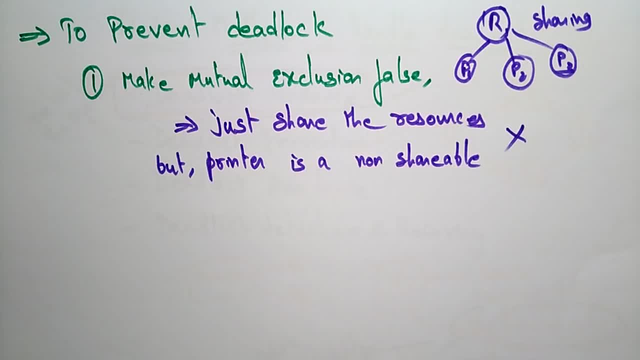 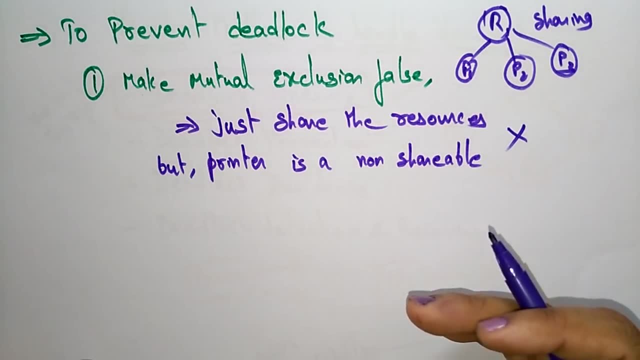 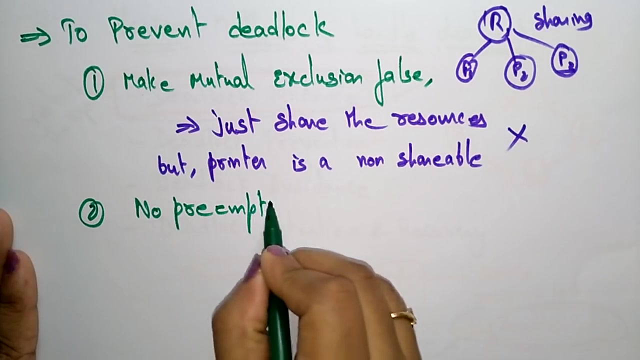 Okay, In some cases you can make mutual exclusion false, But in all the cases you can't make the mutual exclusion false. So this condition may leads to a deadlock and the second thing, so so, so for some cases we can't make mutual exclusion false, just like a printer. so, second is: no preemption, no preemption, try to make no. 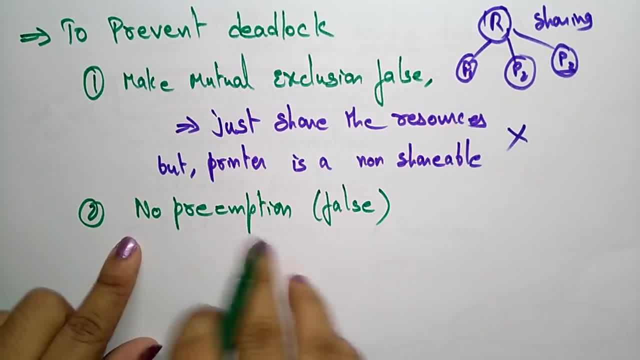 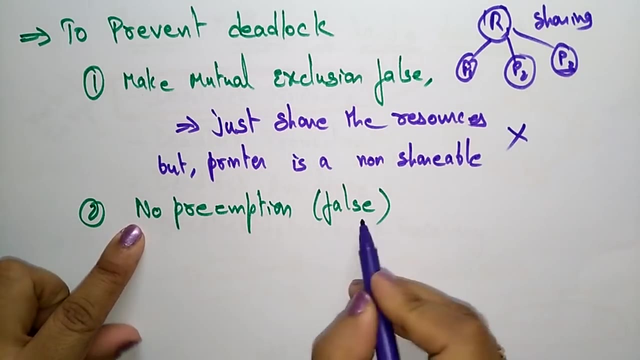 preemption false. try to make to prevent deadlock. try to make no preemption false. so is it possible to make preemption false? so if you want to try to make a pre preemption by using no preemption, false means the opposite is preemption is true. 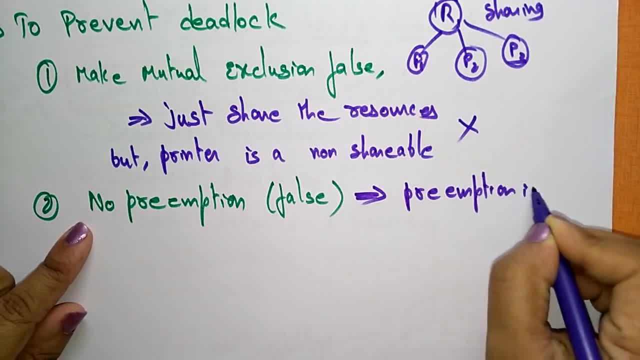 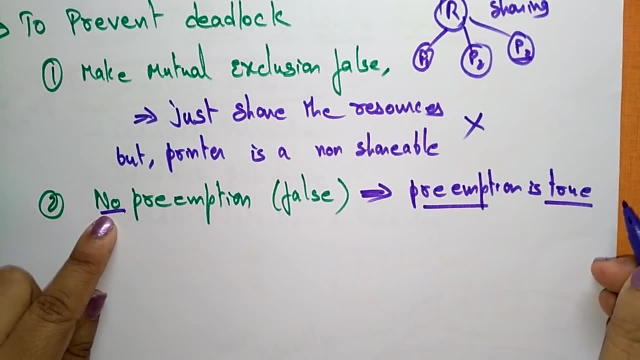 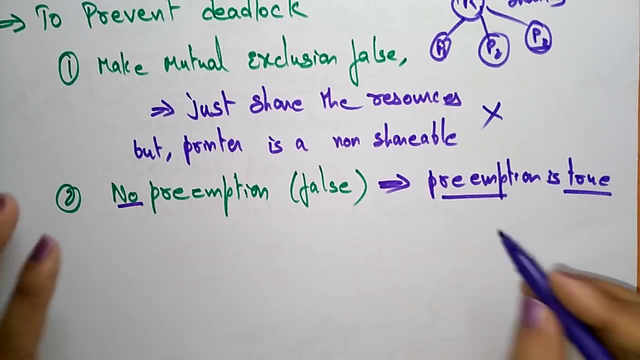 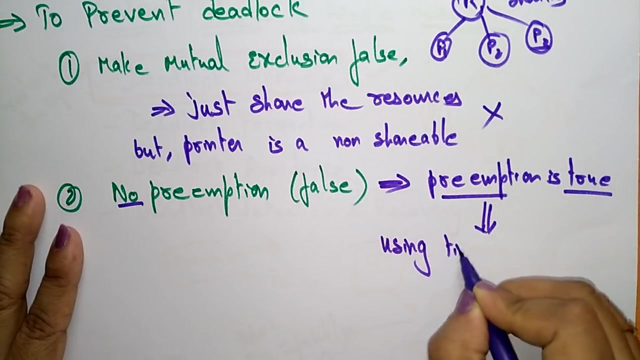 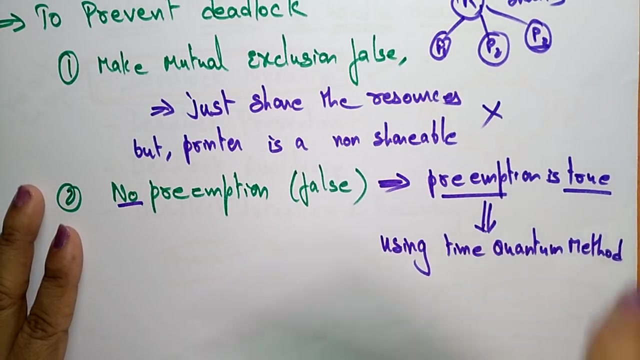 preemption is true. no preemption is false. preemption is true. okay, if you make this preemption is true, then you can prevent the deadlock. so how can you make this preemption true? by simply using time quanting, using time quantum method. so, by using time quantum method, i can make preemption true. 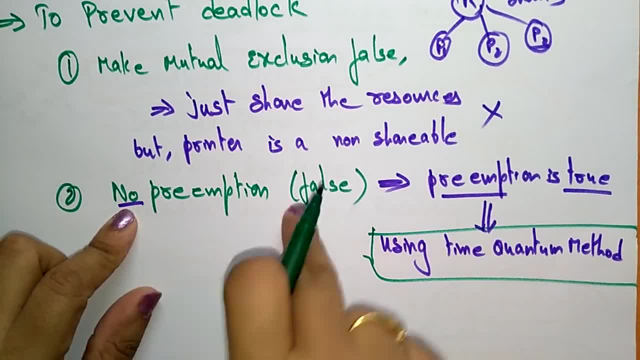 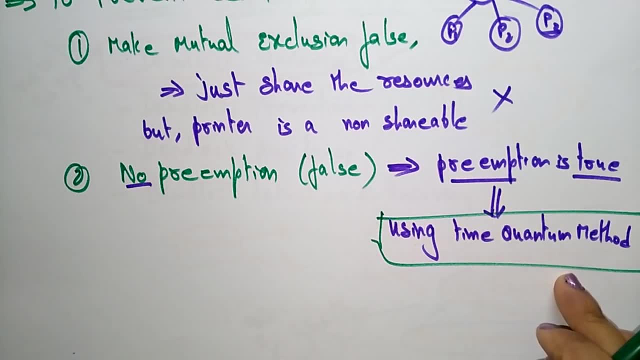 preemption true means obviously no preemption becomes false. okay, so the preemption can be true by using time quantum method. so so what is this time quantum method? here we are allocating time to each process, so the p1 is allocating some time and p2 is allocating some time to access the resources, to access the 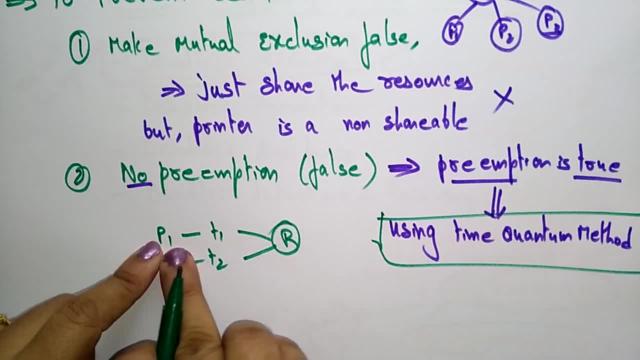 resources. we are allocating some time to process. so whenever the time is over, it has to release the resources. it can't keep the resources with p1, so whenever the time is over it releases the resources, then p2 will take that resources. okay, so that is. you call it as a time time. 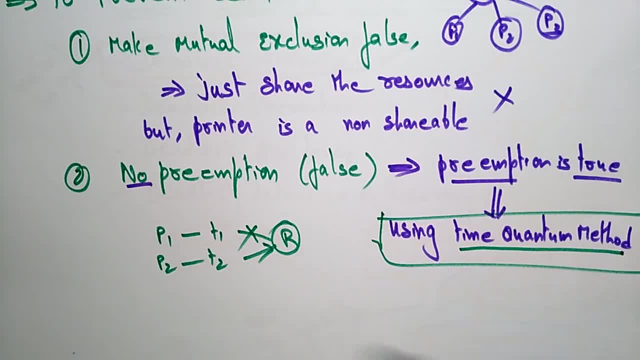 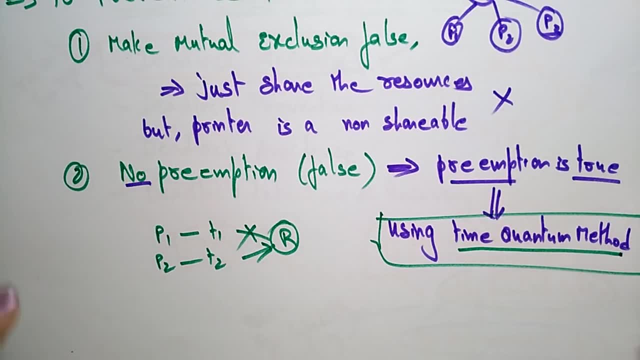 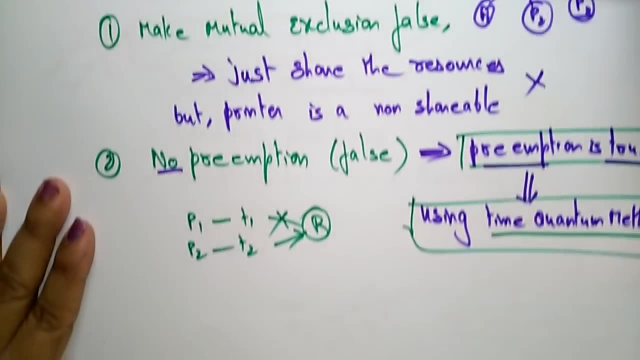 quantum method. so after the completion of the time the resources will be released and another process will take that resources. so so by using pre-emission we can prevent the deadlock. so by using pre-emission we can prevent the deadlock. so next, how we can prevent the deadlock, the third: 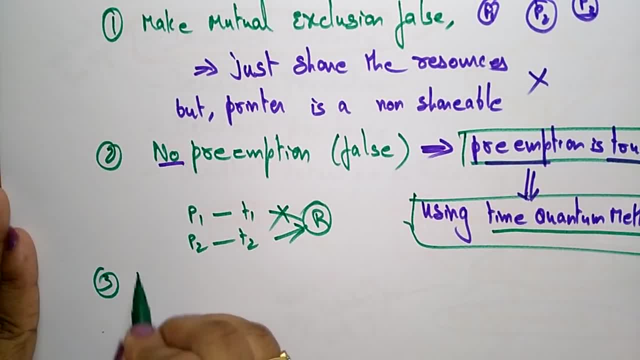 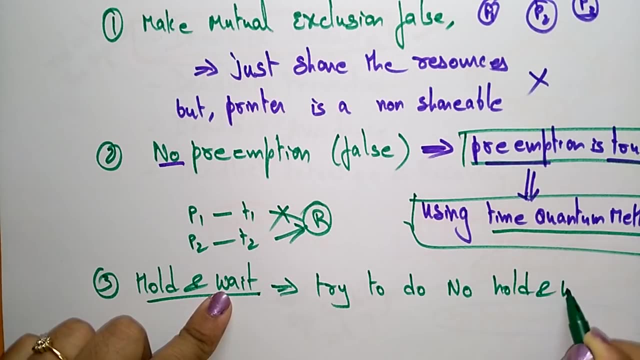 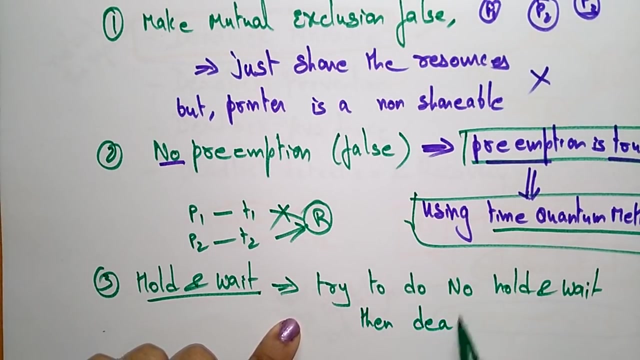 condition is: hold and wait. if you make hold and wait false, how can you make that fold and wait false? by simply try to do no, hold and wait. by simply try to do no and hold and wait, then deadlock can be prevented. deadlock can be. deadlock can be prevented. okay, try to give so. is it possible to? 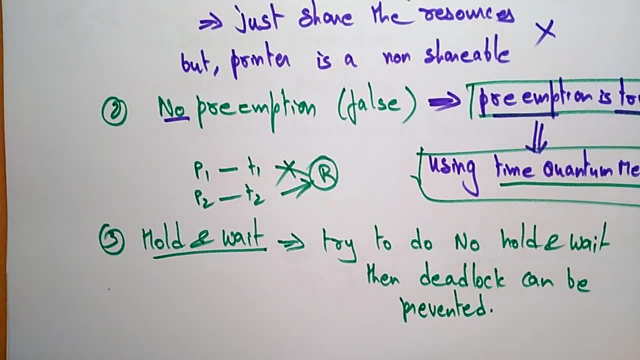 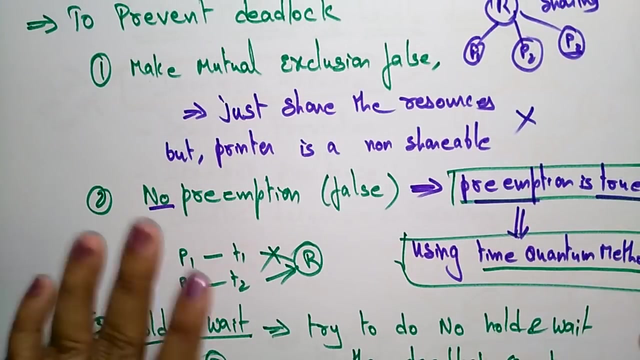 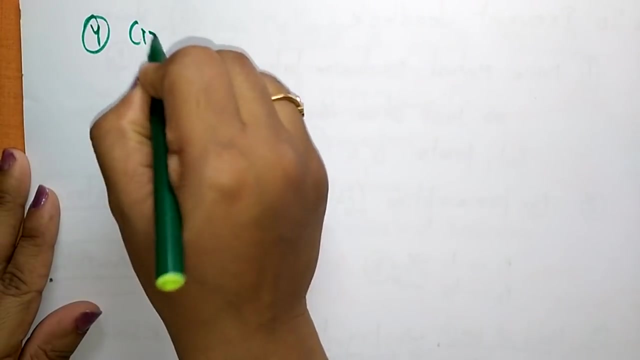 make no hold and wait. yes, it is possible. how can it possible? it's possible to make no hold and wait. yes, it is possible to make no hold and wait. first you try to send give all the resources to the process before it starts. just simply give all the resources to the process before it starts. so then it takes any one of the resources and give it that resource back so that you call it as a no hold and wait. so try to give all resources to the process before it starts. just simply give all the resources to the process before it starts. so then it takes any one of the resources and give it that resource back so that you call it as a no hold and wait. so try to give all resources to the process before it starts so that can be avoid, prevent the deadlock and the fourth condition. so that is a circular weight. so try to make no hold and wait. so try to give all resources to the process before it starts so that can be avoid, prevent the deadlock and the fourth condition. so that is a circular weight. so try to make no hold and wait. so try to make no hold and wait. so try to make no hold and wait, so try to make no hold and 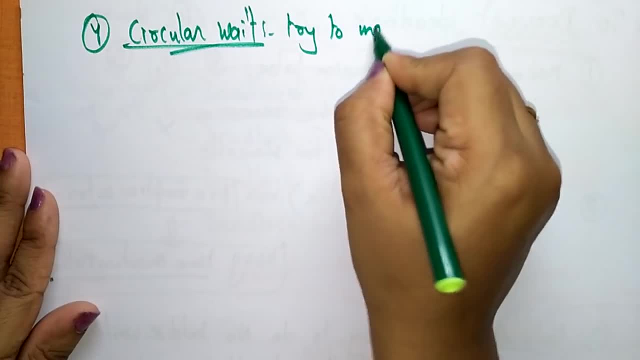 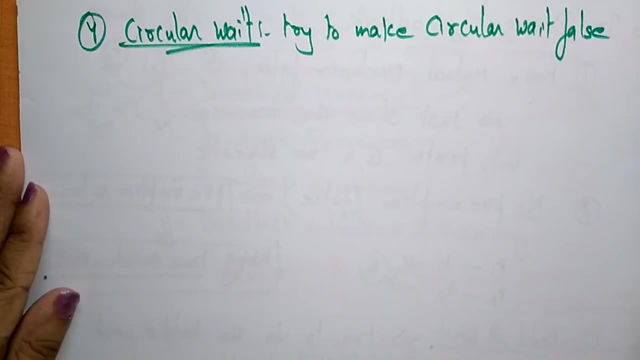 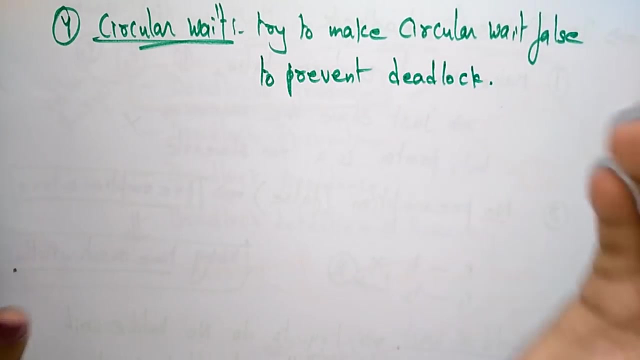 make circular weight false. Try to make circular weight false. Is it possible to prevent deadlock? To prevent deadlock, Is it possible to make circular weight false? Yes, you can make it By simply numbering all the resources you can prevent to remove circular weight. Let me write. 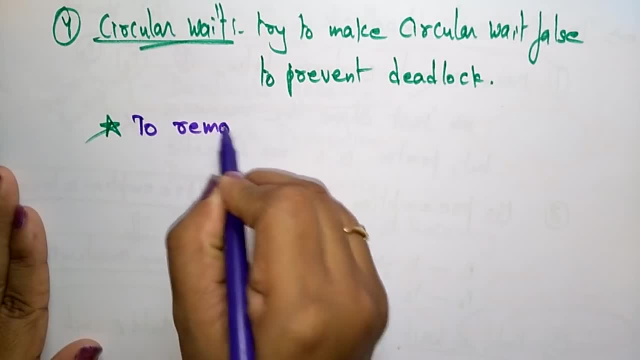 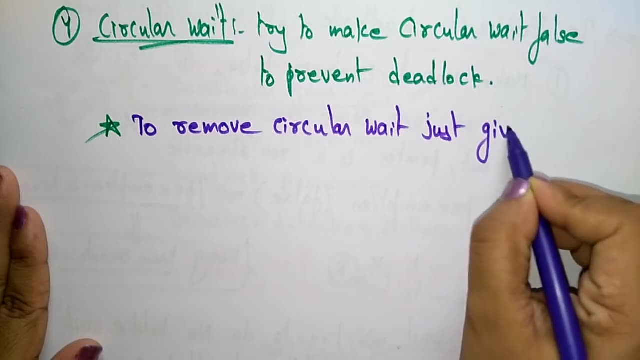 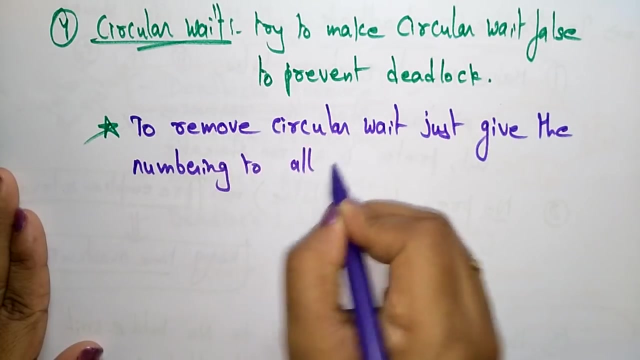 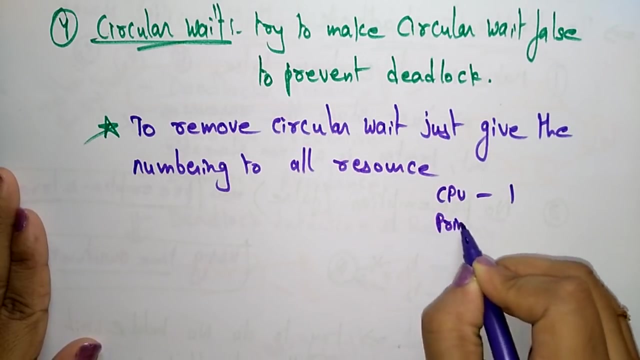 those points, then you will understand. To remove circular weight, just give the numbering. Just give the numbering to all resources. You just give the number to all resources. So suppose the CPU is 1,, printer is 2, like, or else the scanner is 3..